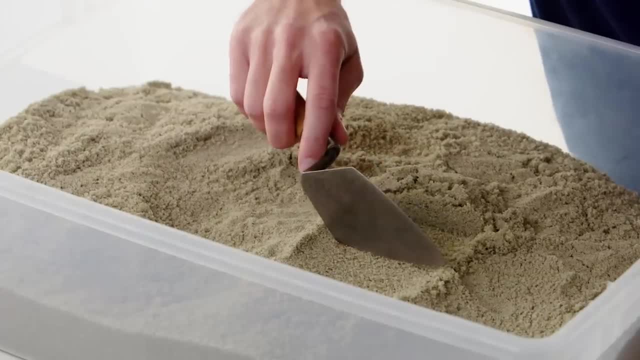 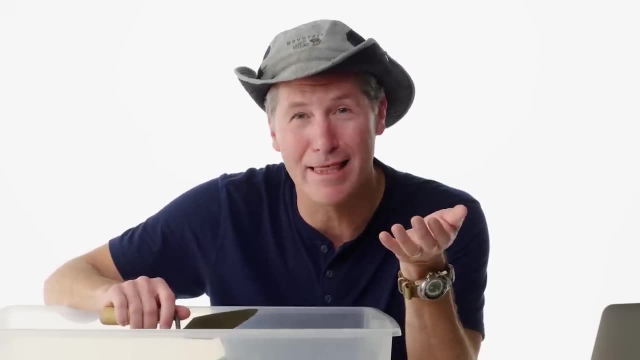 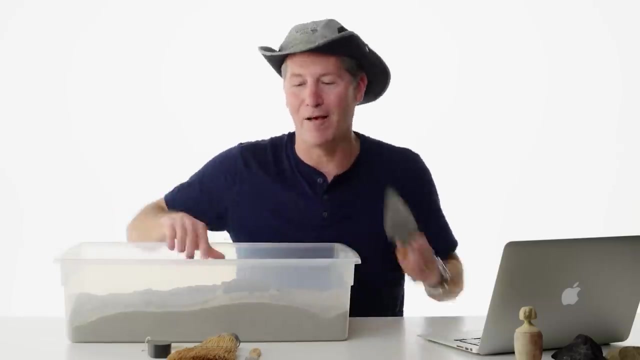 You can dig. You can be really fast with the long edge of it or you can be really precise with the pointy tip. Archaeology is much more about touch sometimes than you would think and sound. You could hear a little clink. Time to slow down. So I take the trowel, put it down, bust out the brush As I brush. 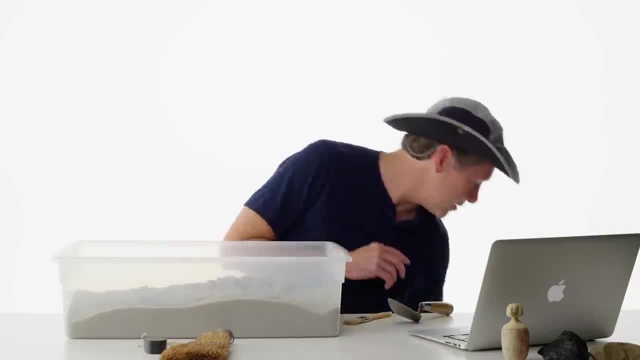 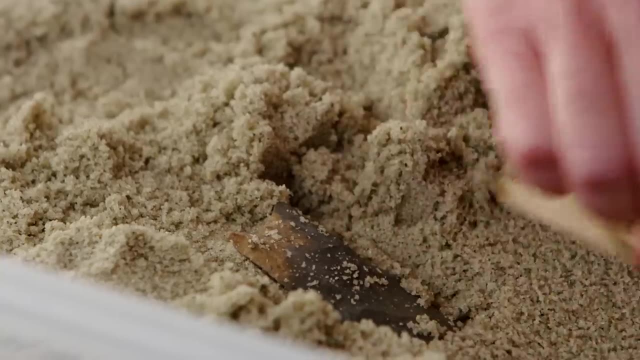 we can see the artifact. At that point we can switch to the popsicle stick. I can push and you don't have that metallic clink. What we would do at this point: pedestal the artifact. We would dig around it. We can say the artifact is 10 centimeters deep. 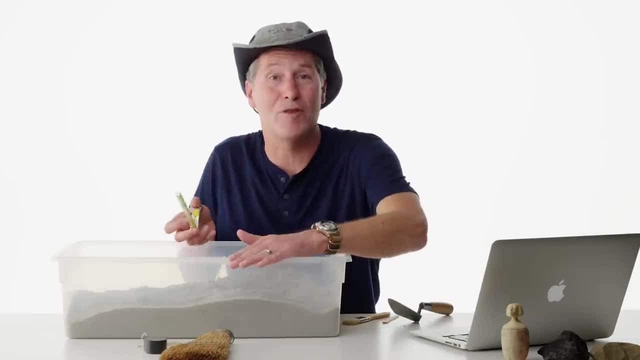 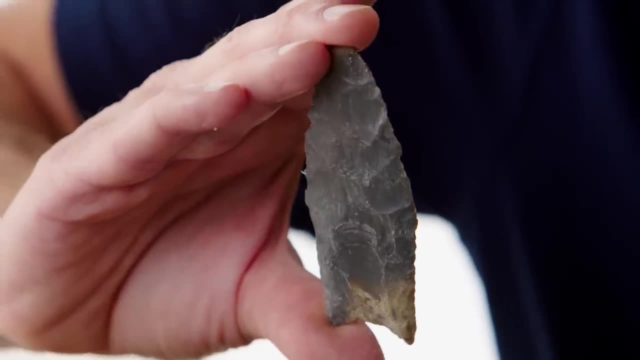 20 centimeters from the west wall, 17 centimeters from the north wall, and then we have the artifact's exact location. This artifact is called a Clovis point, a very specific tool to some of the first people to ever enter the new world. 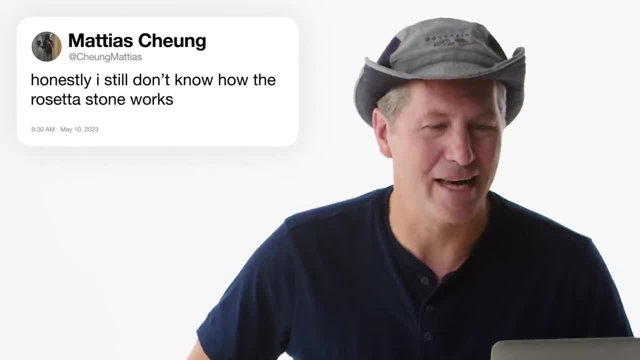 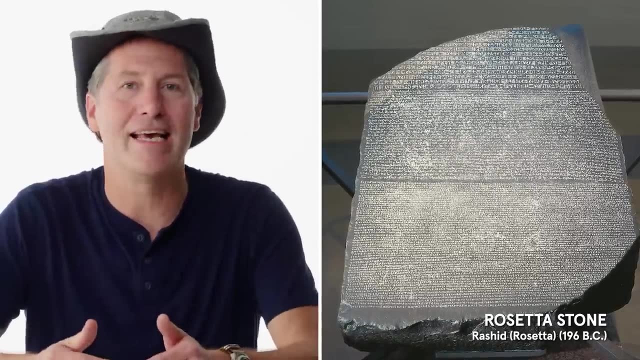 Atchung, Matias asks. honestly, I still don't know how the Rosetta Stone works. The Rosetta Stone is one of the most important archaeological discoveries because it led to to the cracking of Egyptian hieroglyphics. Rosetta Stone was found in 1799 by Napoleon's 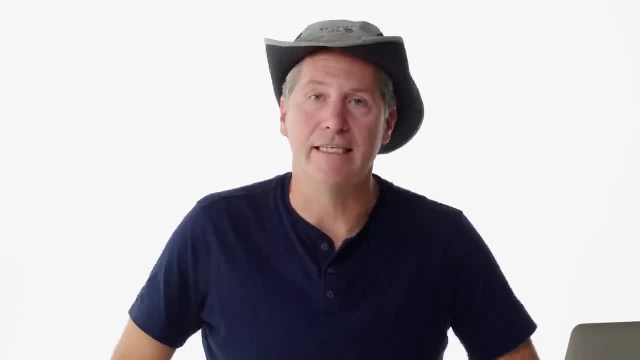 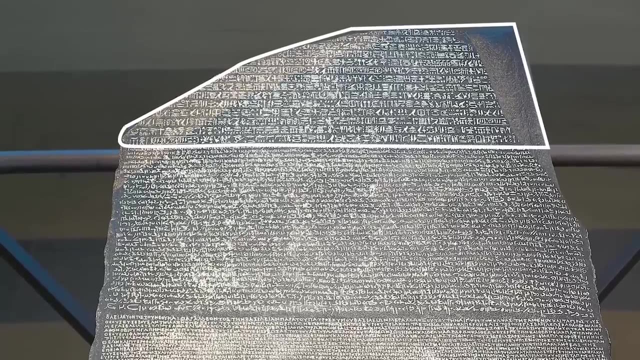 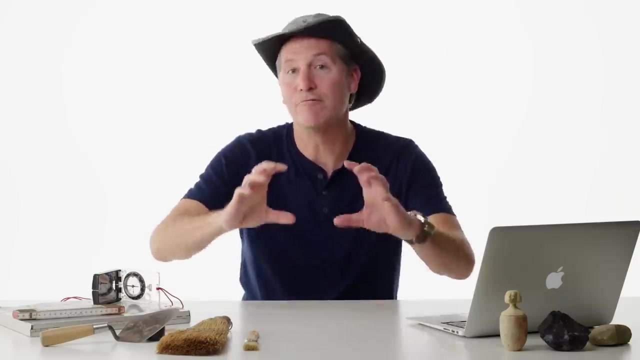 science team that he brought with him in the town of Rosetta in Egypt. What makes it so important is because it says the same thing three times: At the top it's in ancient Egyptian hieroglyphics, In the middle it's in Demotic And at the bottom it's in Greek. So you have this one piece that you 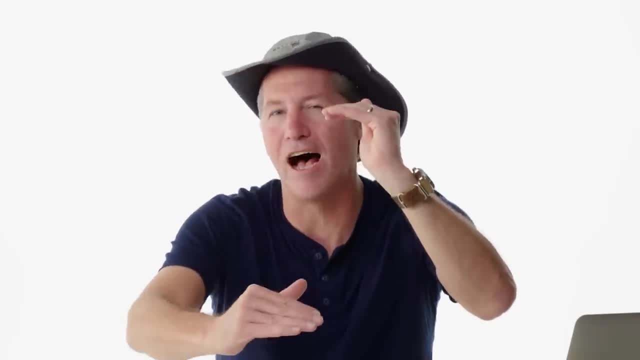 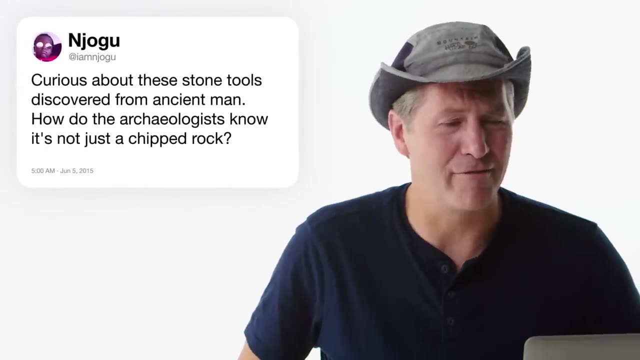 can read, and then you sort of have a key where you can start to build off of and figure out what different symbols mean. And IamNijoju asks curious about these stone tools discovered from ancient man. How did the archaeologists know it's not just a chip rock, If this just 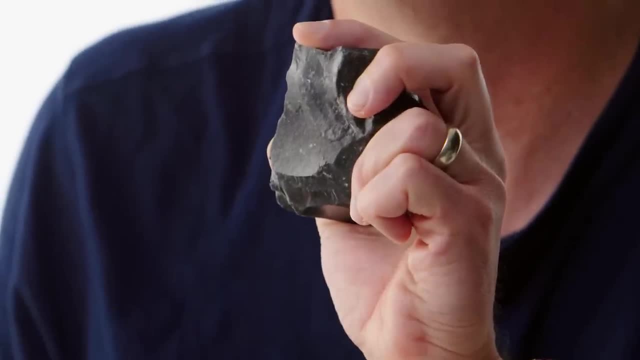 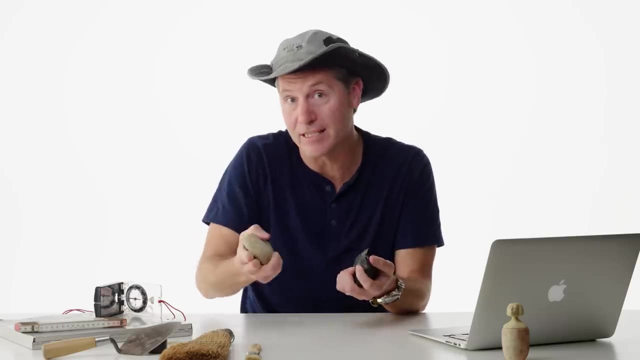 rolled down a hill, it would look different. If I'm an ancient tool maker and I'm using a hammer stone on this, I'm going to hit it really hard to get a flake to pop off. It's going to create what's called a bulb of percussion. It's going to create this divot Also. 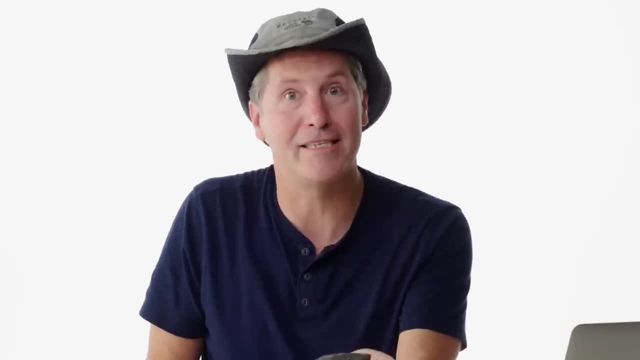 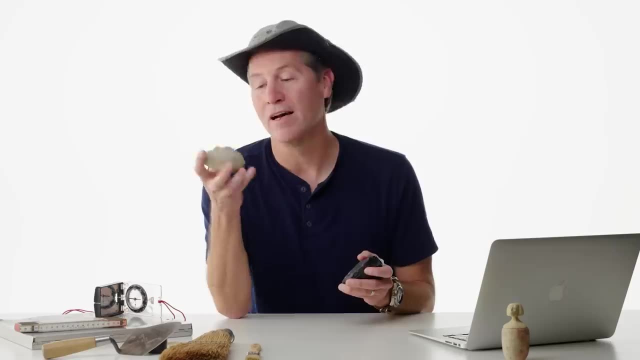 in terms of ancient stone tools. they're going to use things like obsidian. It's volcanic glass. Those types of stones can make a really, really sharp edge. On the flip side, this is a hammer stone. It was very specifically sought after by ancient people. 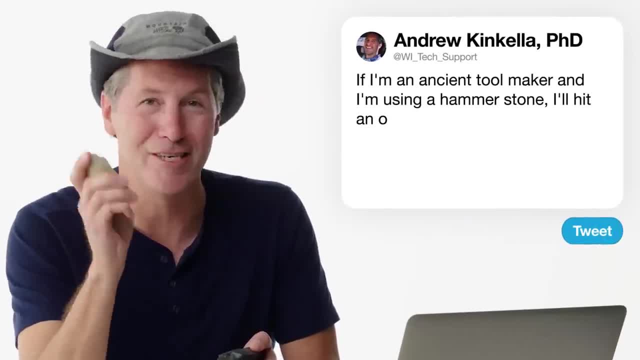 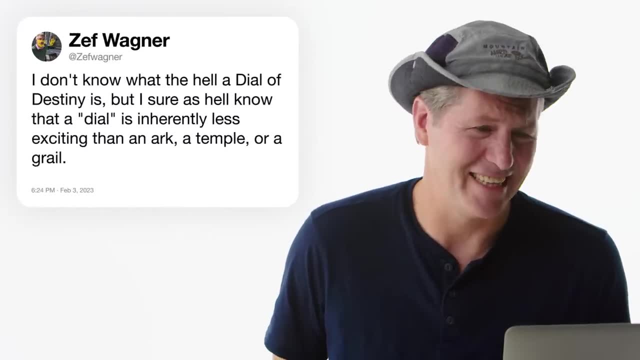 for its qualities of not being too soft or too hard, And you can use it to make good stone tools At. ZefWagner asks: I don't know what the hell a dial of destiny is, but I sure as hell know what a dial is inherently less exciting than an ark. 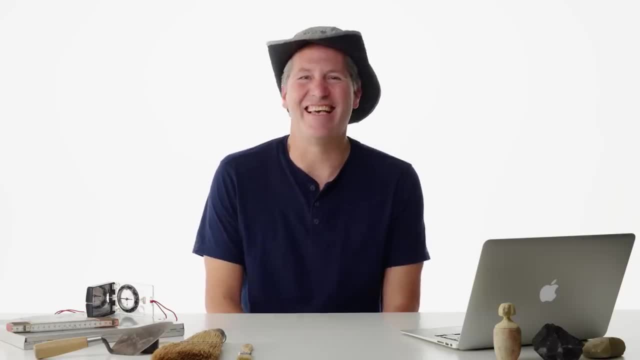 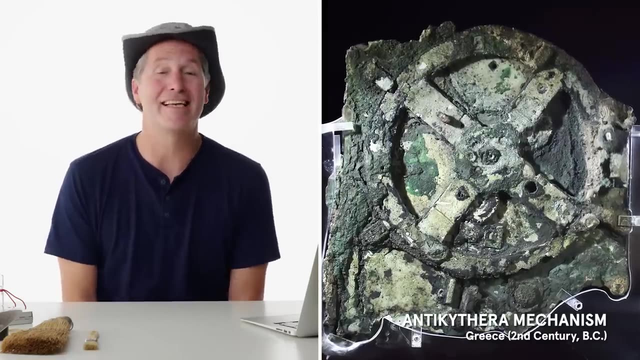 a temple or a grail. The dial of destiny is the new artifact that they're going to use in the new Indiana Jones movie. What they're relating this to is something called the Antikythera mechanism and its ability to track the rotation of planets over time. 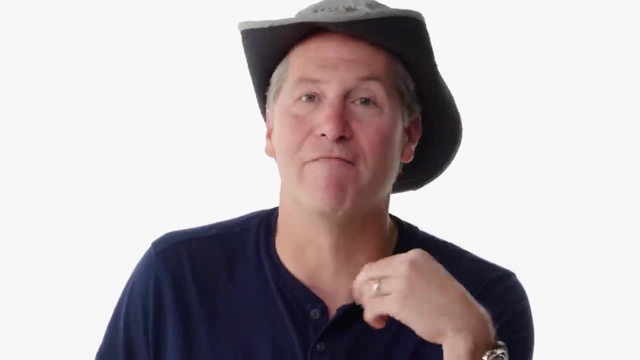 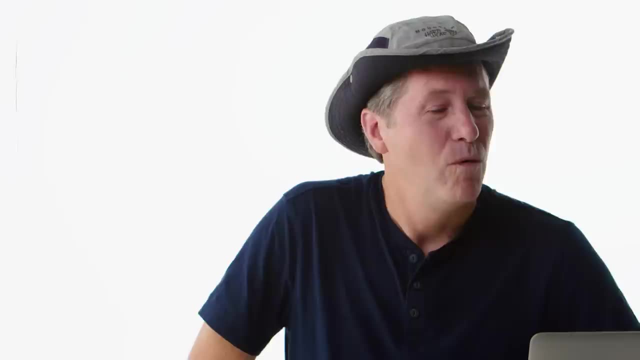 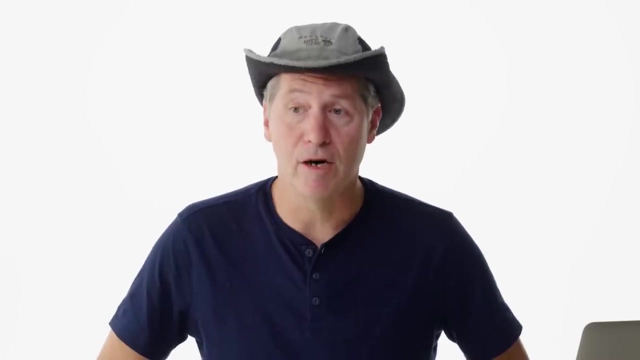 I think what it really shows is an excellent use of math to make the gears so precise that it could at least work for a while. At A-Tang by, Leah asks: why do archaeologists excavate graves again? Sometimes we come across them and we don't expect it. I will say that is the most. 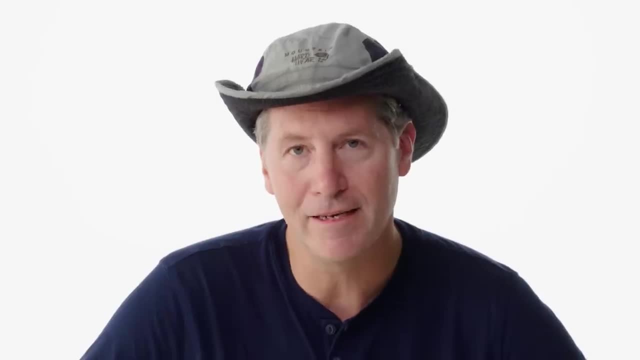 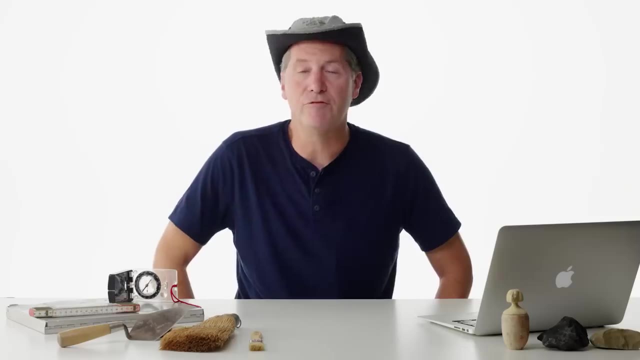 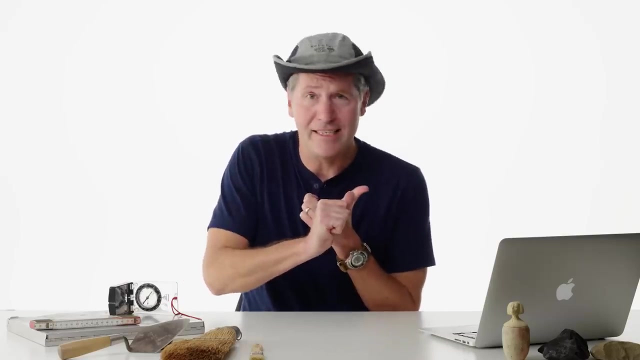 common way that we find human remains. It's a little bit of a deep moment. You do start to think about your own mortality. Human remains that you find in a grave tell you so much about the past. The human skeleton itself can tell you how that person died. Did they have any diseases? 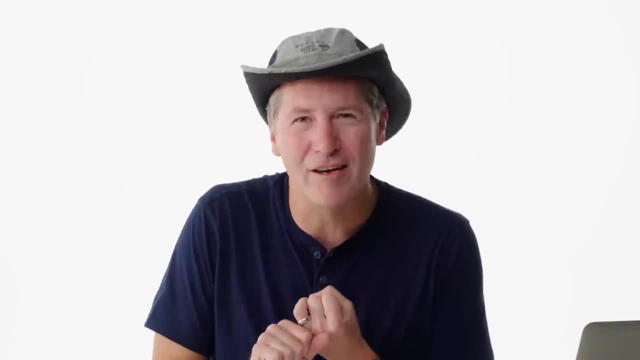 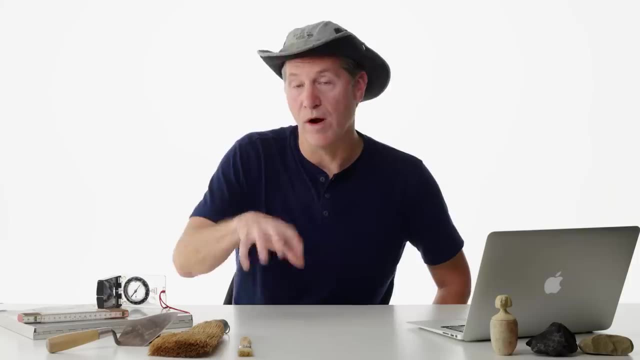 What was their social status? It can tell you about the religion of the culture. When we excavate something like a human burial, we go very slow. We work with local communities. Where are you going to store these? Where are you going to store these? Where are you going to store these? Where are you? 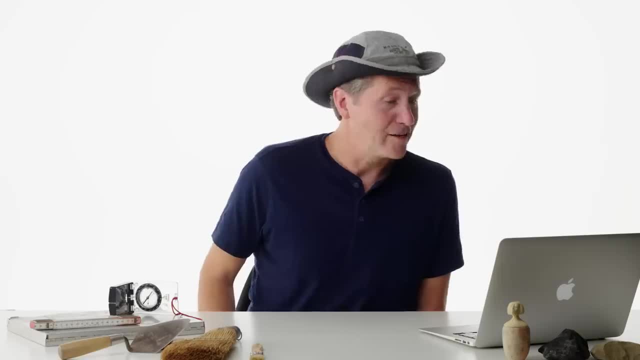 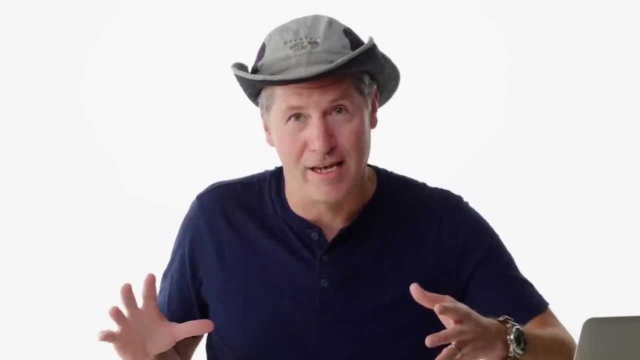 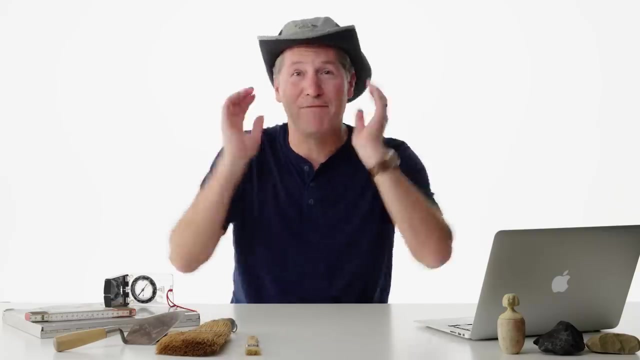 going to bury these human remains? Are you going to rebury these human remains At Gough? Logan asks: how does this carbon dating thing work? Carbon-14 is an isotope. It breaks down over time And what we can do is measure the rate at which it breaks down. Let's say, after I'm filming this, I walk off. and I die in the parking lot, My carbon-14 starts to go down. 5,730 years from today, I will have half as much carbon-14 as I have carbon-14.. I will have half as much carbon-14 as I have carbon-14.. 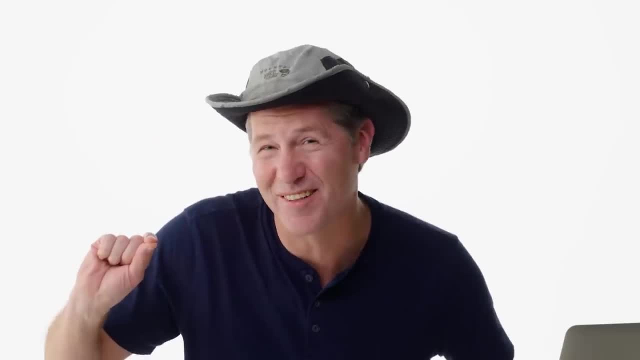 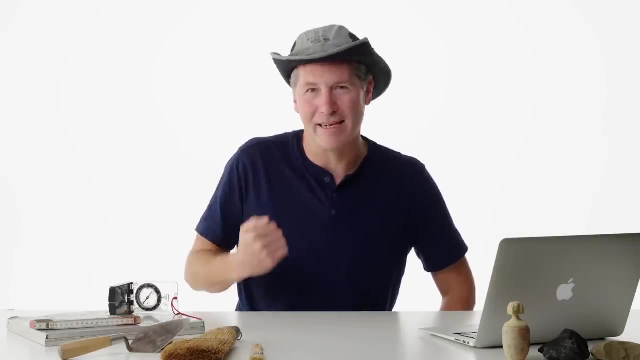 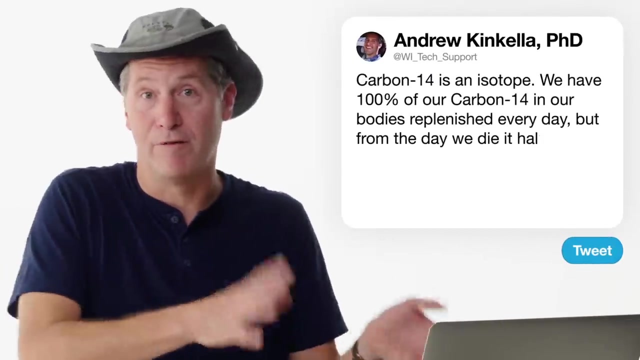 I will have half as much carbon-14 as I did in the beginning. Now, if you add another 5,730 years, I have a quarter of what I had. Now you got to watch it because it only works on things that were once alive. You cannot carbon-14 date a rock, But for living things- burials- remains. 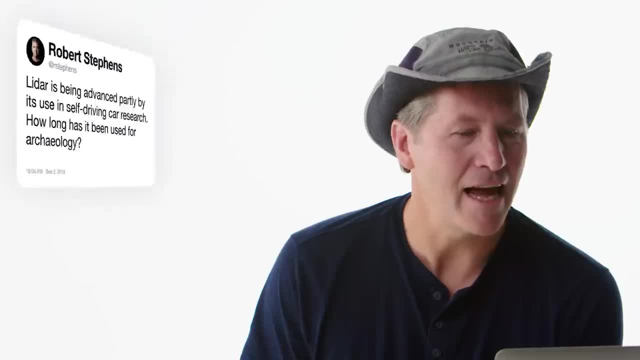 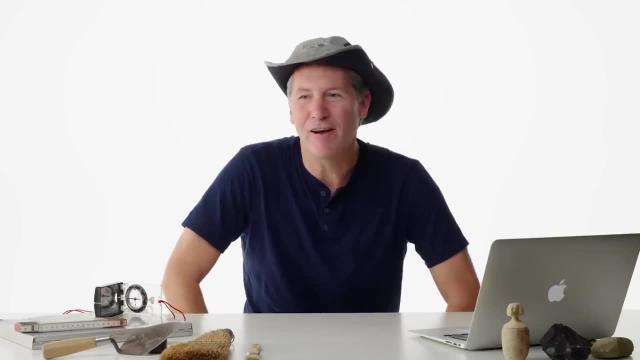 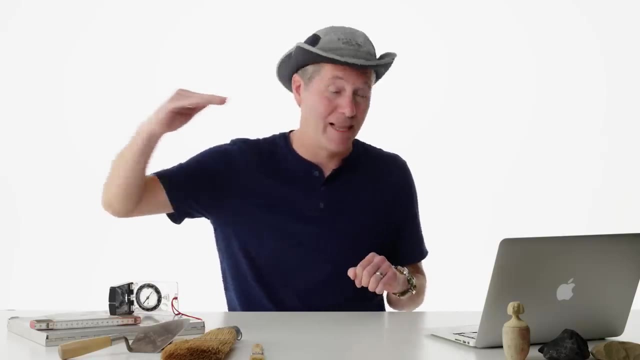 we can get a date for it At. R Stevens asks: LIDAR is being advanced partly by its use in self-driving car research. How long has it been used for archeology? It's been used in archeology the last 10 years or maybe more. But LIDAR is a bunch of lasers shot down from a plane or a. 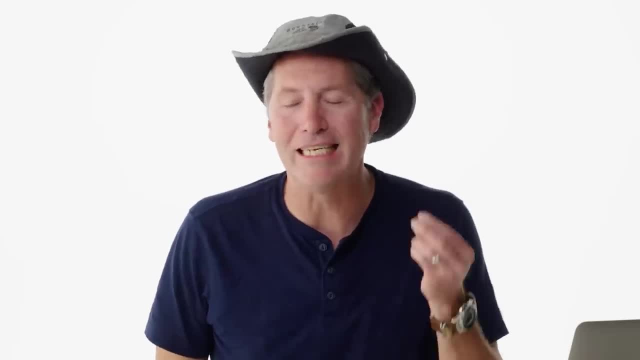 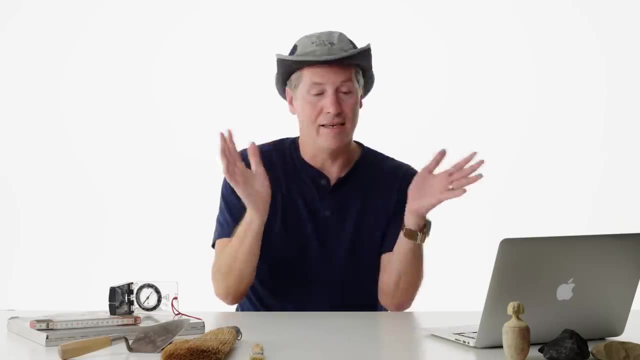 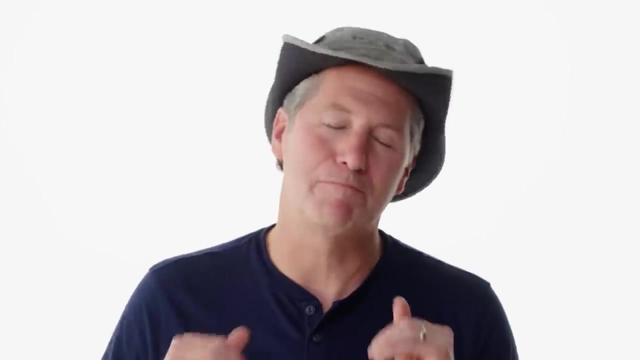 helicopter that flies over a site. What it gets is really, really specific geographic and mapping data. So as the plane flies over and shoots a bunch of lasers, the trees actually blow a little, So a couple of the laser beams will get down to the ground surface. It used to be just prohibitively. 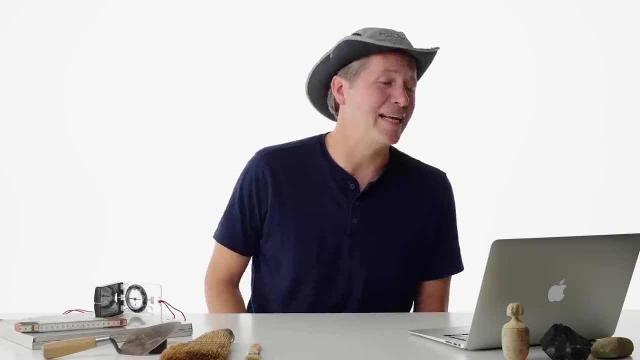 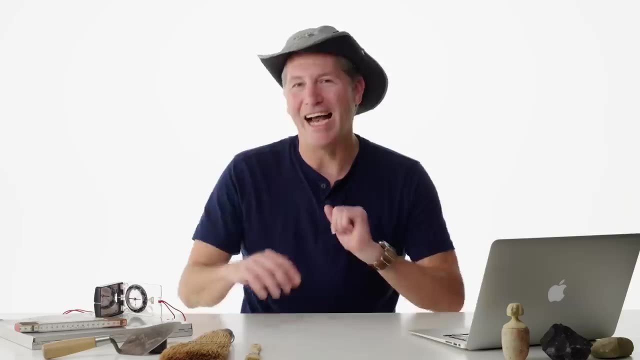 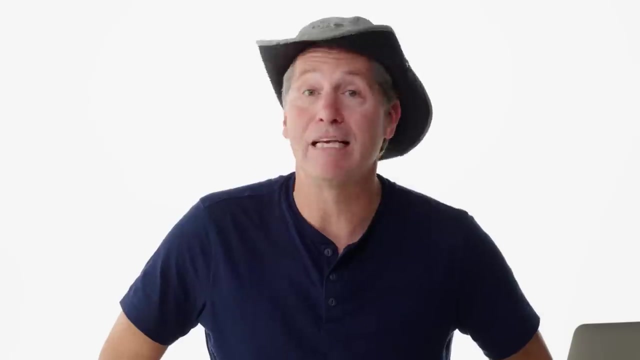 have it due to the decreasing cost At Bryce. P Wrights asks: how often do archeologists have to think: are these bones a crime scene or a discovery? I did once work on a salvage archeology project where a construction crew had accidentally hit a family plot. that was about 80. 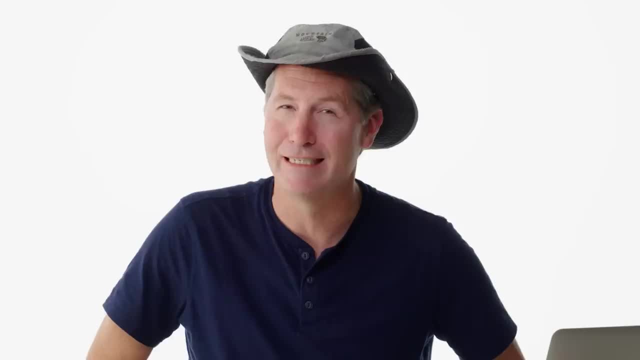 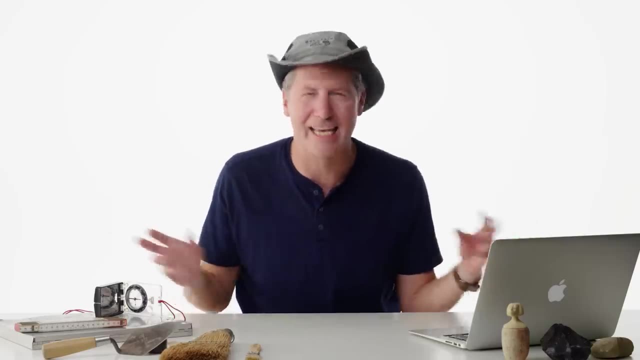 years old. The skeletal material was still kind of supple. You can really tell the difference if you're working with something that's thousands of years old, because it's totally dry and it started to kind of wither away. So they're not bleach white like you would think They're. 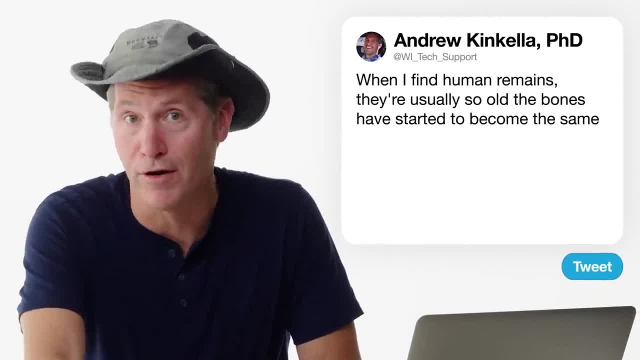 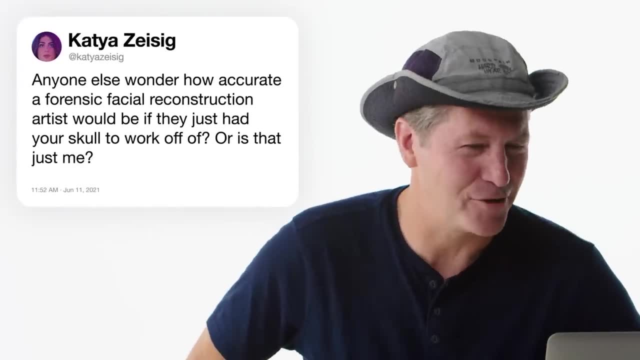 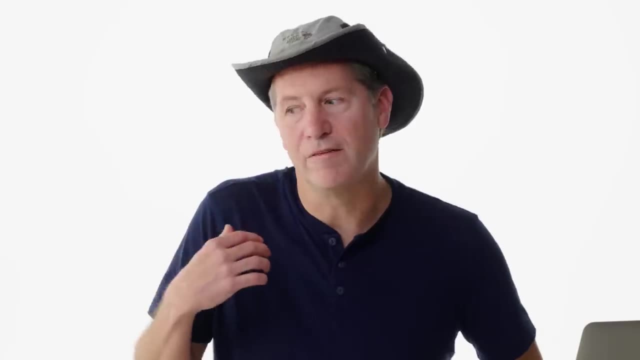 sort of a dull brown. I still will call the coroner just to make double sure. At Katya Zizeng asks. anyone else wonder how accurate a forensic facial reconstruction artist would be if they just had your skull to work off of? We have to realize that it's not perfect In terms of facial 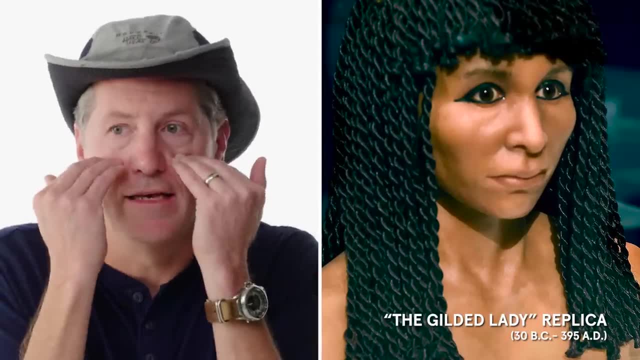 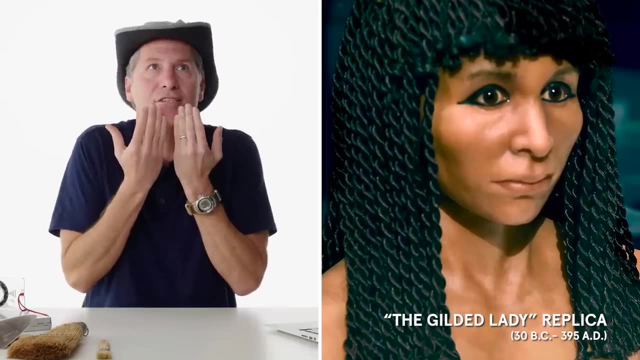 reconstruction from a skull. some things you can get are stuff like the cheeks. Are the cheeks higher or lower? The eye sockets? Are the eyes higher or lower? Are the eyes higher or lower The eye sockets? the brow ridge, the chin, the teeth. Sometimes the chin will be more of a jutting. 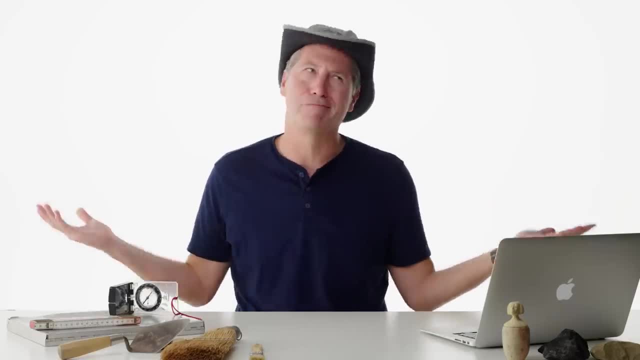 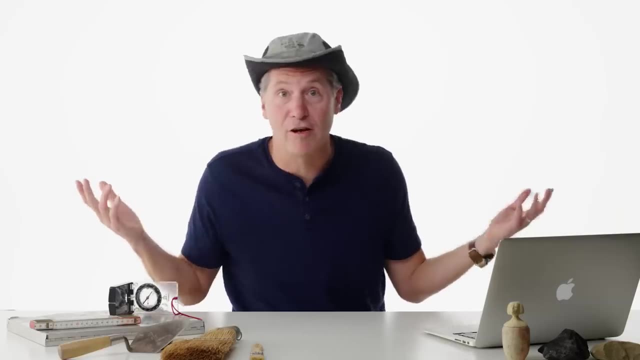 chin, but stuff like what was the overall shape of the nose, you know the ears, You're going to go with the trends of the time. So if you're working on a skull that's 4,000 years old and it's a male, 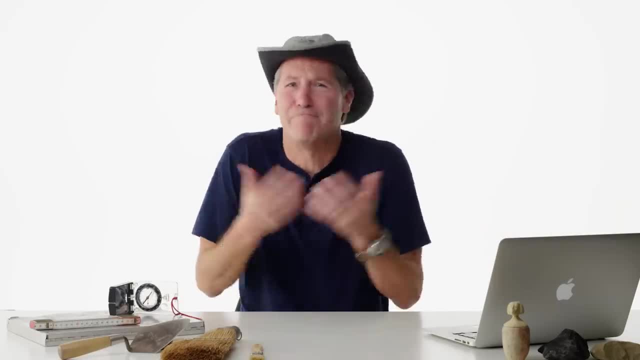 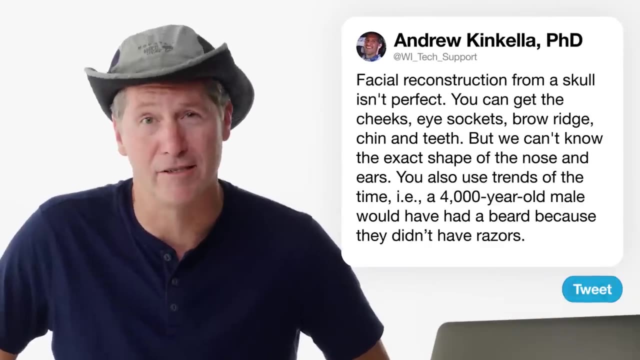 skull. you're going to put some sort of beard on it because they didn't have Bic razors 4,000 years ago. Archeology is literally three pieces of the thousand piece puzzle At Malachi. Waters asks: do I have to be a human? I don't have to be a human. I don't have to be a human. I don't have to be a. 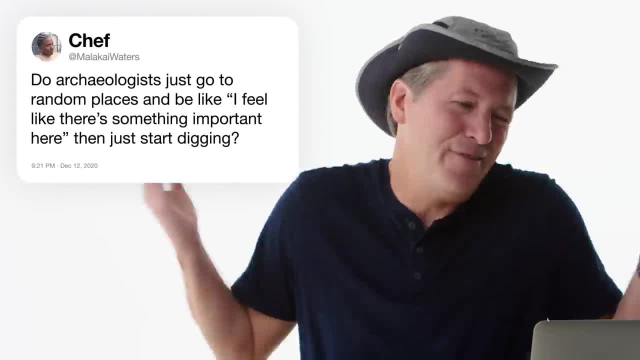 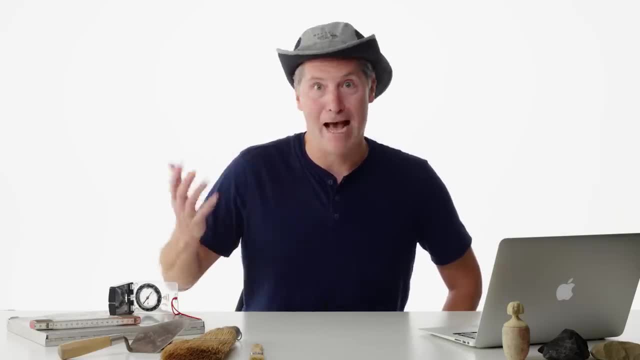 human. Do archaeologists just go to random places and be like I feel like there's something important here and then just start digging? We only excavate after we've surveyed and mapped the location. We are looking for the best possible places that archaeological sites might exist. 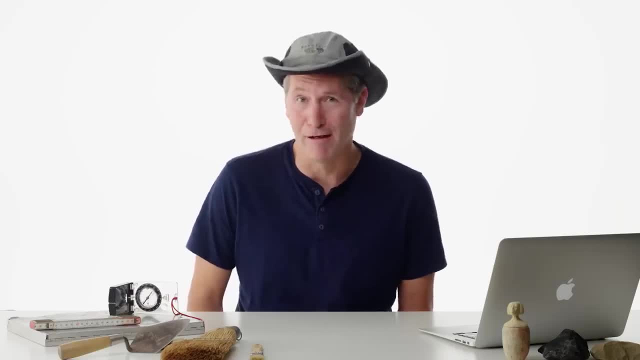 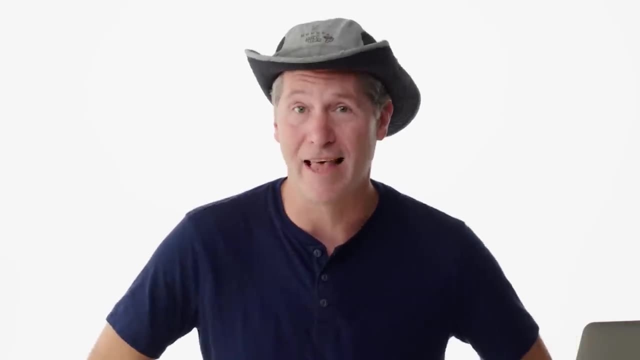 The ancient Maya would build on good soil. If there's a forestry company or something who has made a map of the soil quality throughout the region, I love getting that map, because that makes my work that much easier. I love getting that map because that makes my work that much. 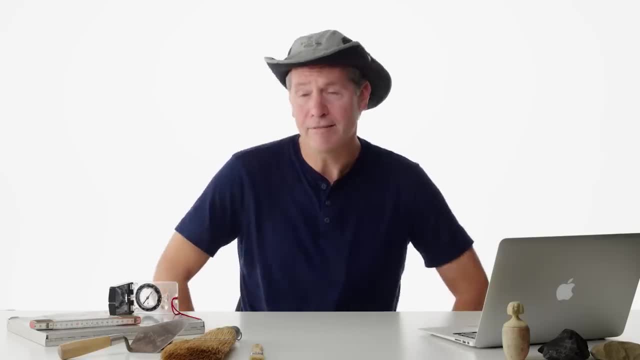 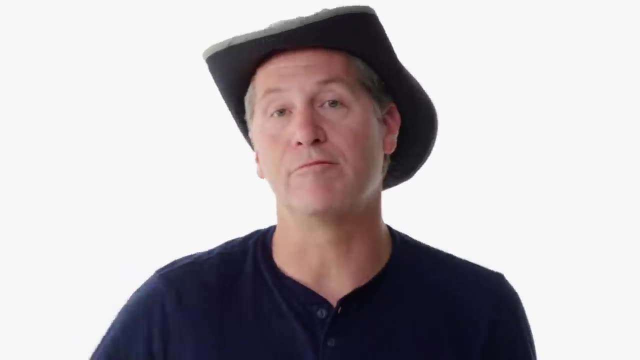 easier. I was working on a project in downtown LA where they were replacing the sidewalk and they took up some of the concrete and there was a human skeleton right there. This was a human skeleton that had been there for hundreds of years. In the modern world we want to have, 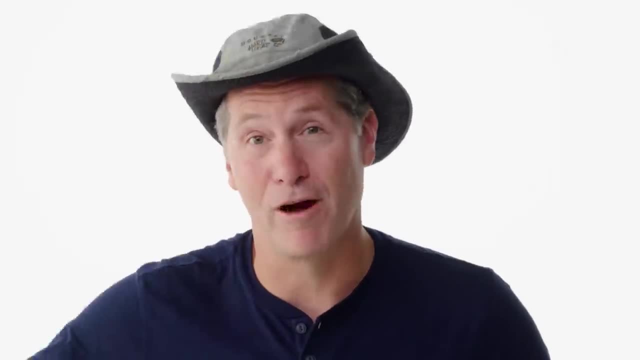 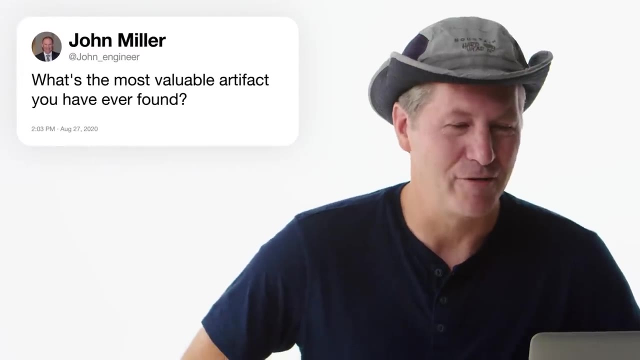 archaeologists along with construction projects and building projects, because they do find things like this from time to time. At John, Engineer asks: what's the most valuable artifact you have ever found? I'm going to go with an entire Mayan pyramid. I found the most valuable artifact I've. 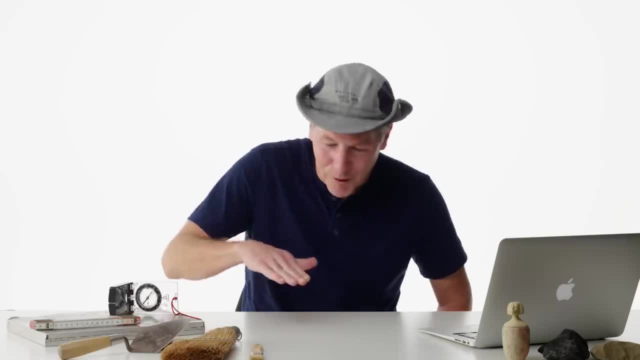 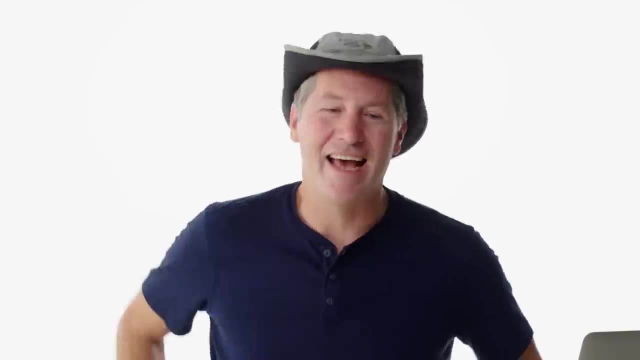 ever found. I found the pyramid through Google Earth at home. I rolled the cursor over this area of the jungle and the altimeter would go bloop, bloop, bloop, bloop, bloop, bloop, bloop And I thought: 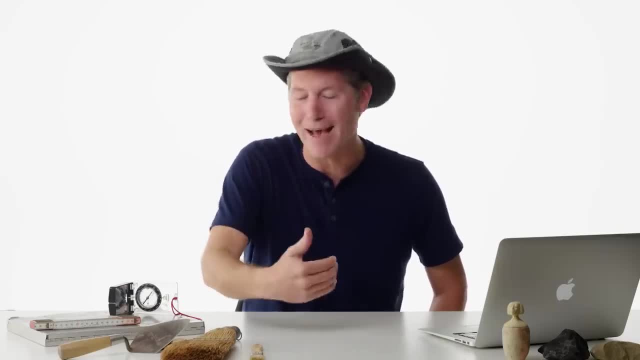 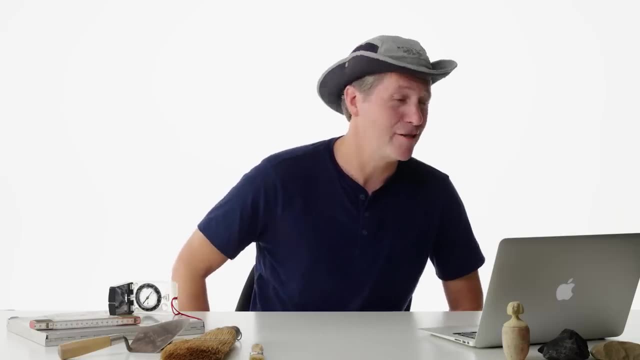 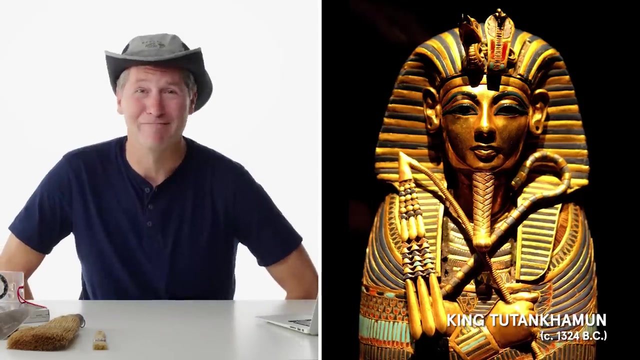 you know, next time I'm in that area of the jungle, I got to go back there and check out that area And, yes, it actually was an ancient Maya pyramid. At Joe Six, Totoro Bear asks: what archaeological find do you wish you had made and why The tomb of Tutankhamun? 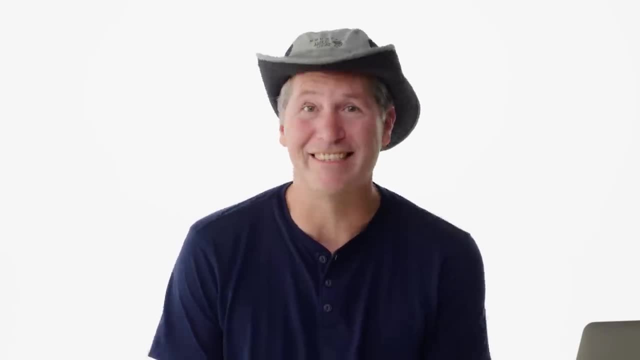 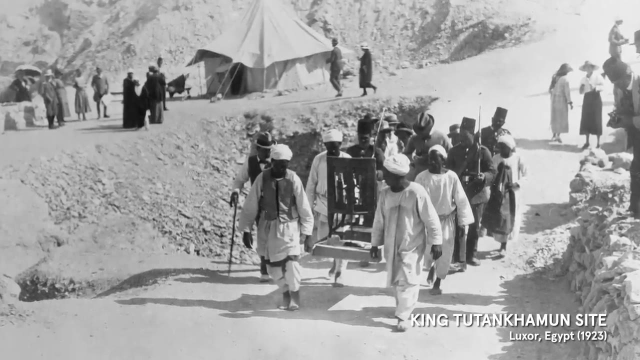 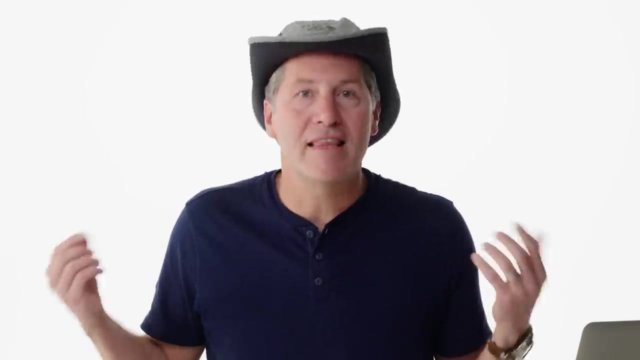 In the early 1920s. it took him several field seasons and he had to look for months through the entire Valley of the Kings at his last little survey square. That's where it was. Those artifacts are amazing- Stuff like wood that's 3,000 years old. It looks like it was. 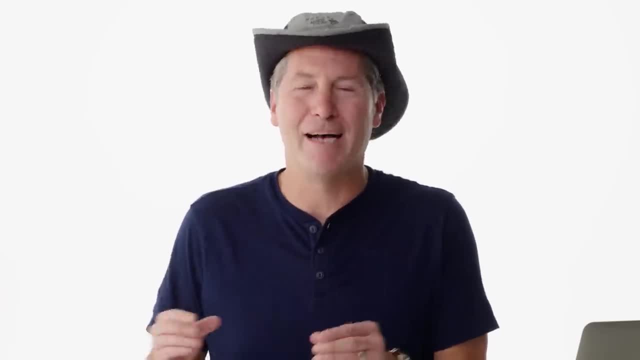 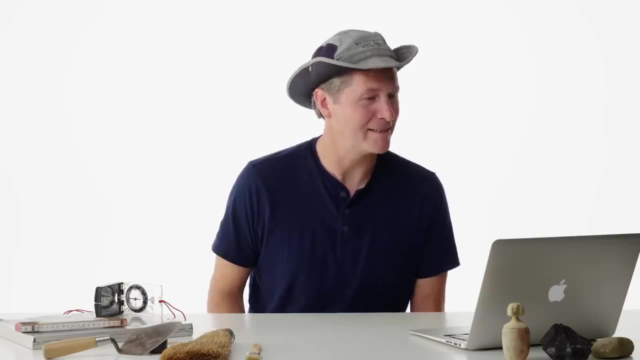 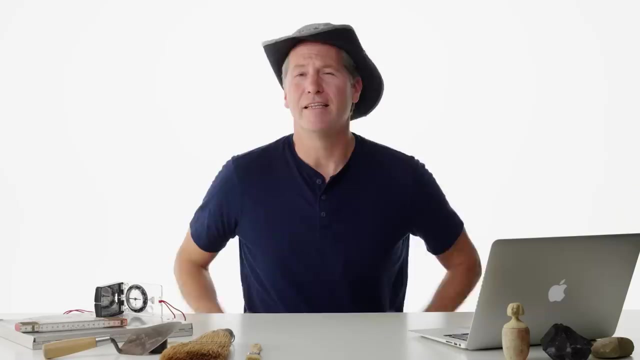 made last week. They tell you so much about this little moment in time when this young king died unexpectedly At Jane Loves Bees asks: do archaeologists even do sex estimations of skeletons? Yes, And it's usually fairly easy. The two best places to look are the skull and the pelvis. For a male skull it tends to be more. 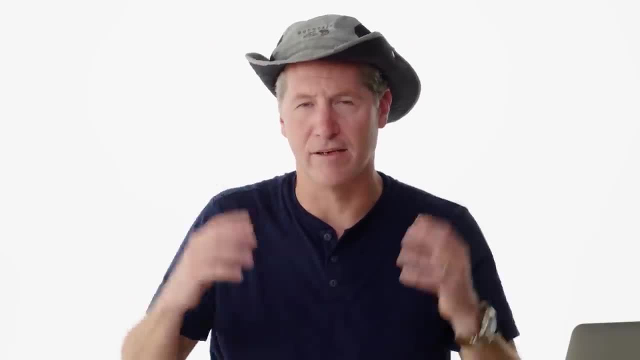 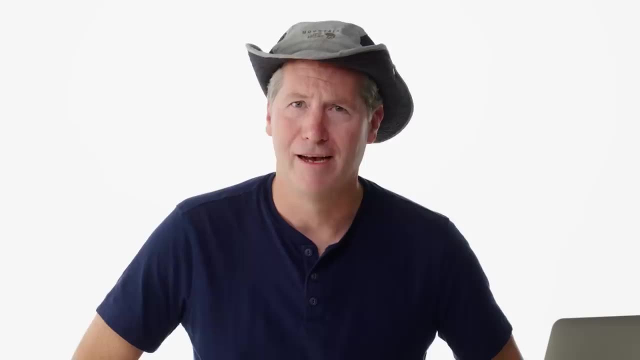 robust. It'll just sort of be bigger overall, a bit more angular, Although there's a lot of overlap on this, So you have to look at different, very specific parts of the skull in order to be sure. I got this wrong. once Now it was a skeleton that had no head. The pelvis looked very, very 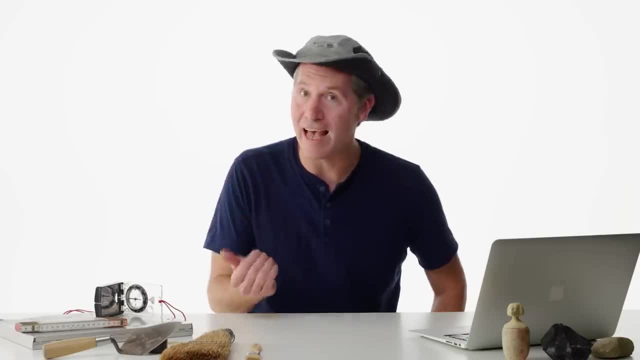 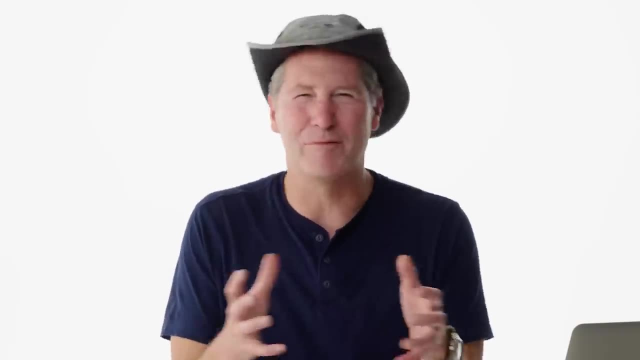 narrow And I was like it's a guy. Once they got it to the lab and they could look more closely, it was a female who had a very narrow pelvis. In the field there's still parts of it covered with mud. It's in a bad position, But once it's in the lab it's under controlled conditions. You can. 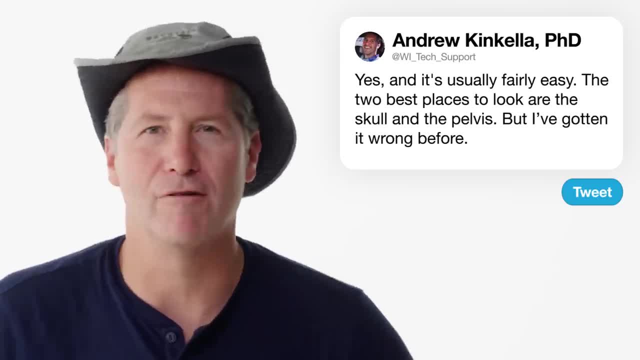 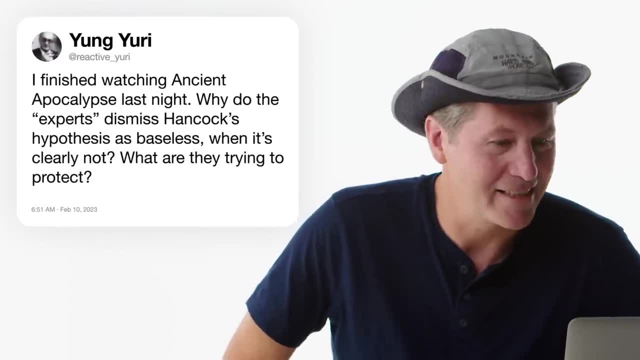 get really exact measurements. You can just get a much better idea of what's going on At Reactive. Yuri asks: I finished watching Ancient Apocalypse last night. Why do the experts dismiss Hancock's hypothesis as baseless? Ancient Apocalypse is a Netflix series. 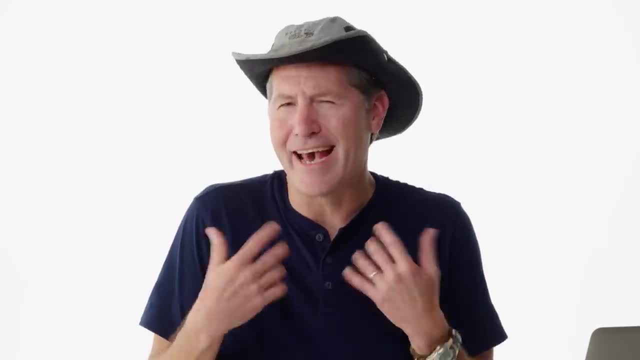 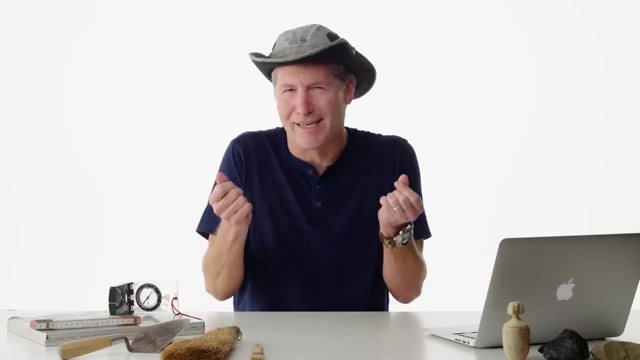 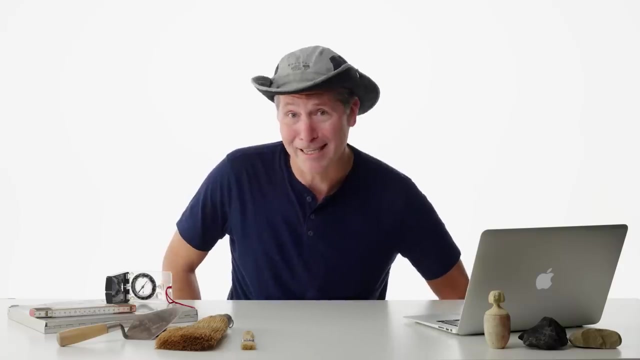 whose central premise is there was a cataclysm about 10,000 years ago that destroyed a super, advanced, super civilization, And we only have bits and pieces of that left. It didn't happen. There is no evidence. One of the best examples of this is the Piri Reis map. It was done in the early 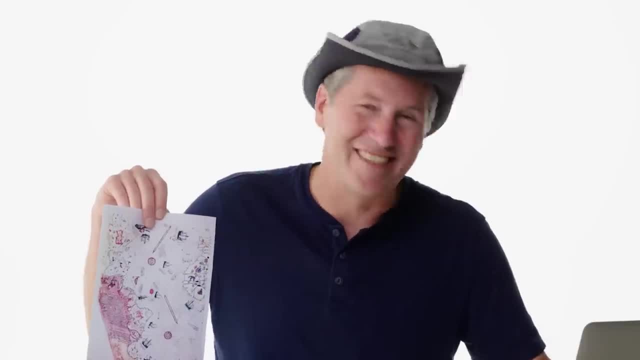 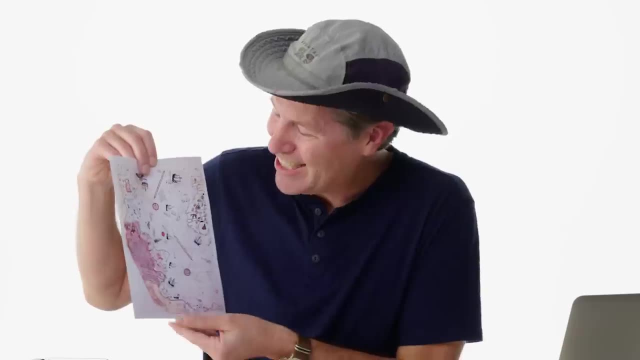 1500s made by this guy named Piri Reis. Pseudo-archaeologists like Graham Hancock say this is evidence that ancient people explored the Piri Reis map. It's just not. It's proof that ancient mapmakers ran out of paper, curved it around. This is just 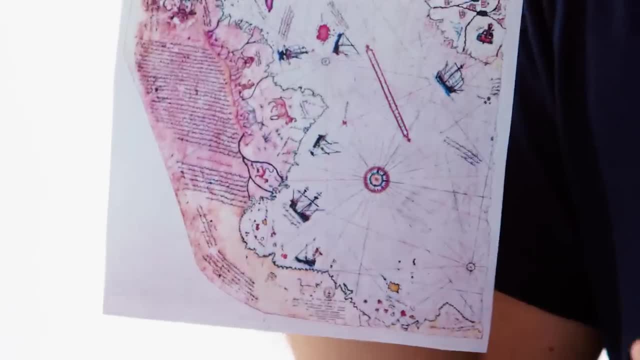 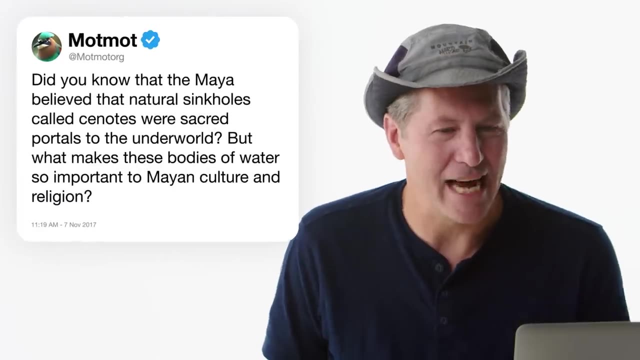 a part of South America. We can't use this today as serious scientific evidence. It's not At. Motmotorg asks: did you know that the Maya believed that natural sinkholes called cenotes were sacred portals to the underworld? I am a Mayanist and I did my dissertation. on the cenotes of Belize. Sometimes they were just used for water, but other times they were used for water. They did sacrifice people into the cenotes from time to time. I don't want you guys to think that human sacrifice happened like every weekend or something. It didn't If the crops were going. 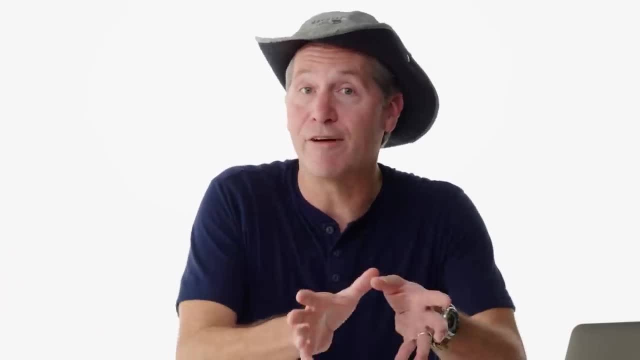 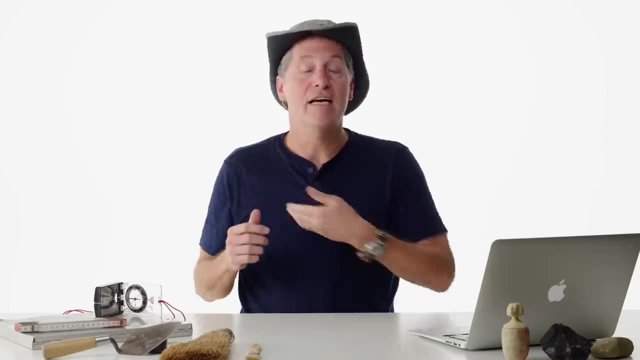 poorly and if there was no rain, you may sacrifice somebody who was usually a captured warrior from one of the other cities. Take this person to the edge of the cenote. You would slash them through their chest. We have found human remains in some of the cenotes. We have accounts from the Spanish 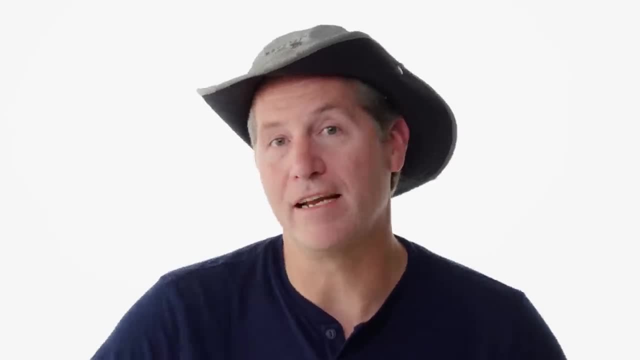 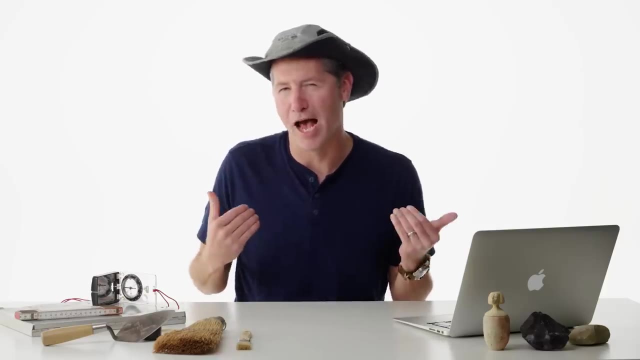 of seeing this kind of thing happen. In terms of my research, we did find a little building right on the edge of the cenote, And we would call that a water shrine, And that would be the place where these kind of rituals would take. 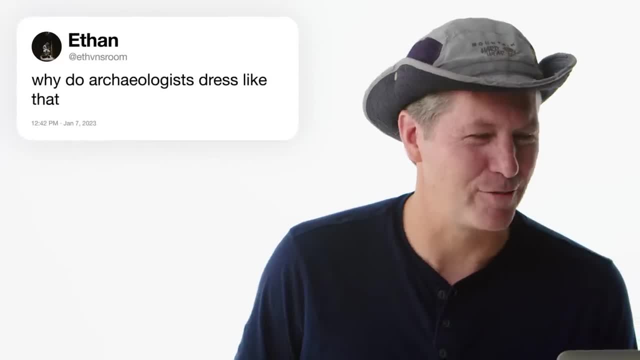 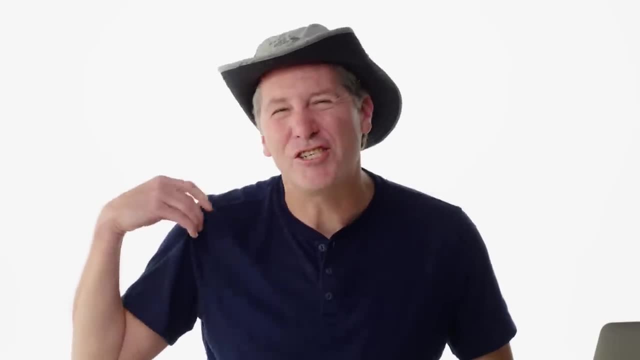 place At Ethan's Room, asks: why do archaeologists dress like that? It depends on the environment. you're working in For me, in the jungle. I'm going to wear a light shirt. I'm going to have boots on. I'm going to bring a machete with me in order to cut through the jungle. I'm going to wear 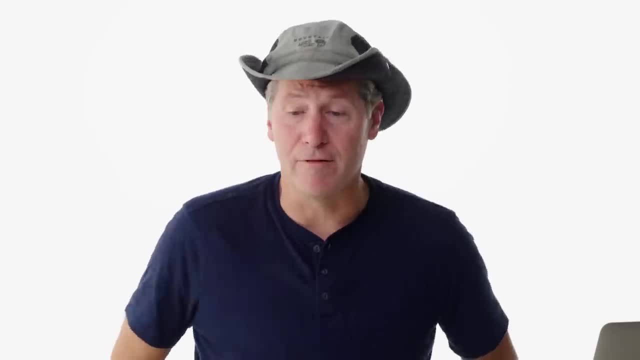 a hat: Protect yourself. I'm going to wear a hat. I'm going to wear a hat. I'm going to wear a hat. You will also bring with you a bunch of different tools in a backpack or a satchel, A GPS unit, If I. 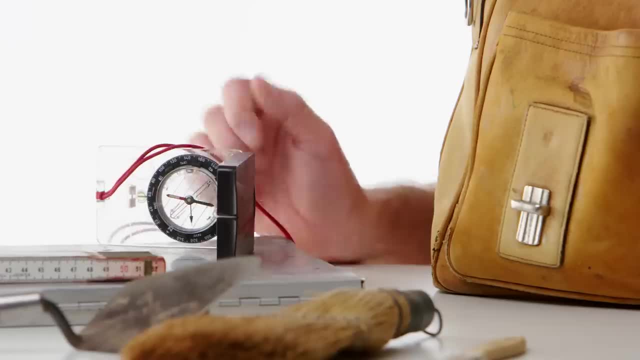 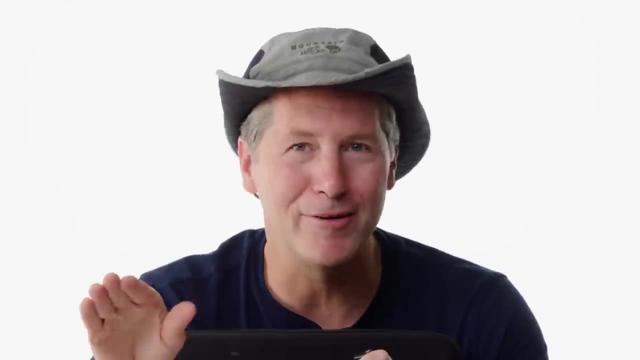 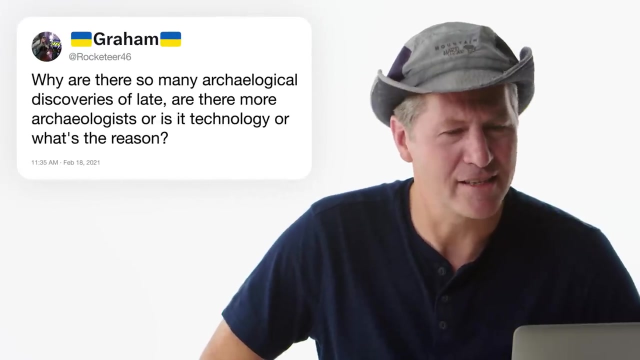 had to bring one thing with me, it would be a compass. The compass will get you home. GPS units are great. They work on batteries And once you're out of batteries you're dead. Always trust your compass At. Rocketeer46 asks: why are there so many archaeological discoveries of late? Are there? 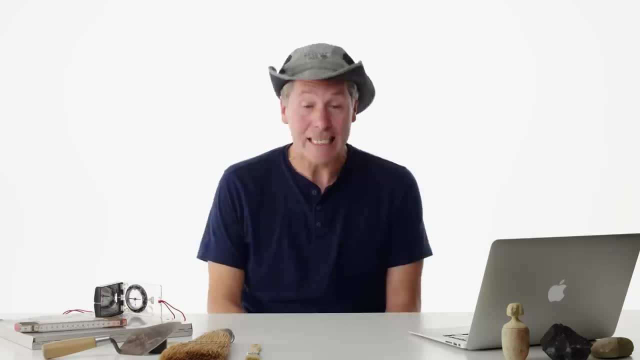 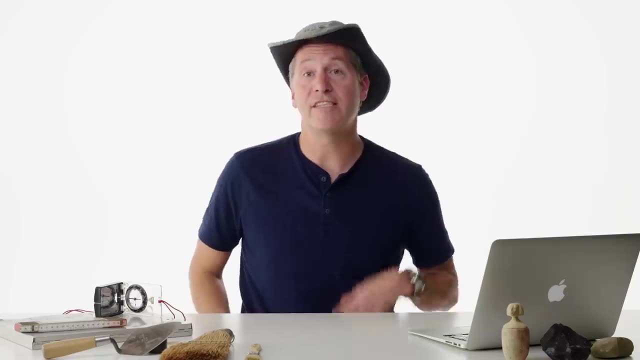 more archaeologists, or is it technology Or what's the reason? It is true that we tend to be finding more and more stuff. We do have more modern technology, like LIDAR. There's also satellite technology that help us find new sites, And we can see things like 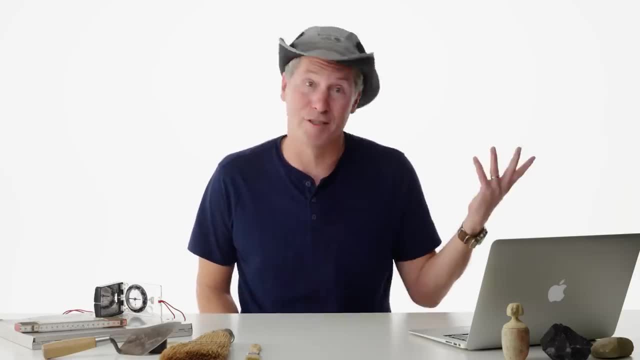 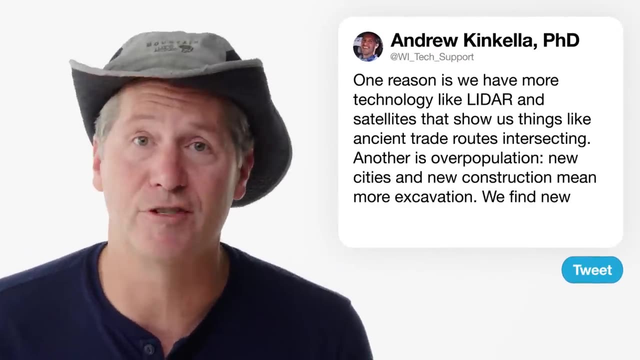 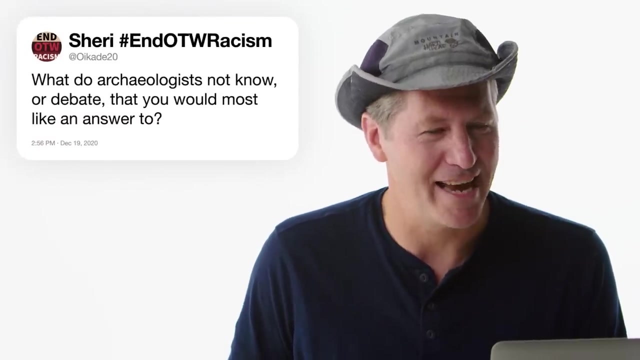 ancient trade routes, But a major part of this is world overpopulation. There is more and more excavation, So we find new archaeological sites in every country of the world. At OikaD20 asks: what do archaeologists not know or debate that you would most like an answer to? 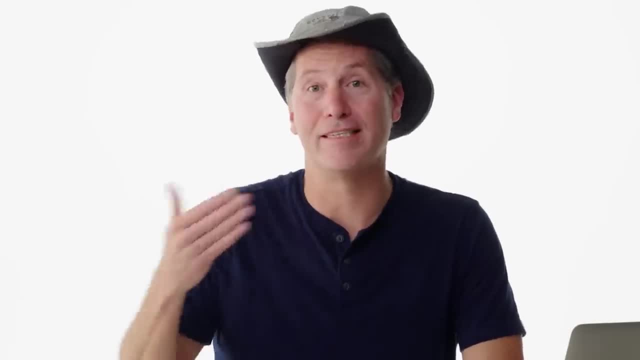 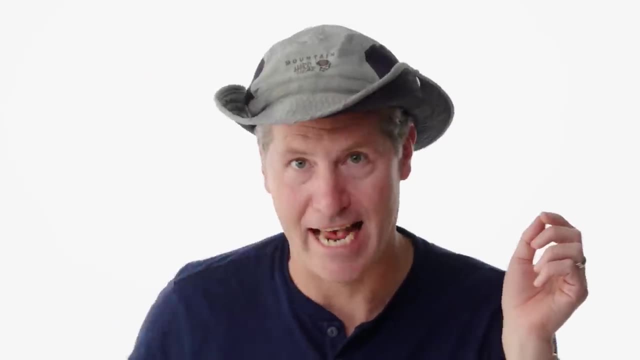 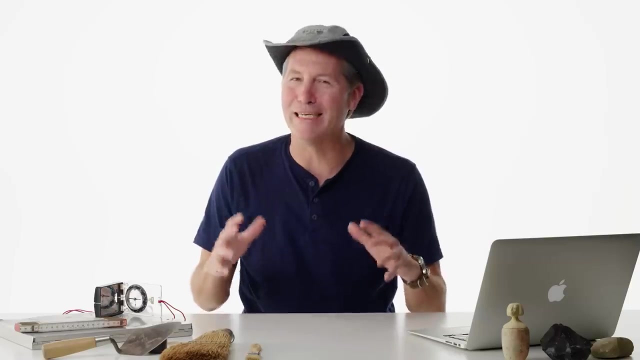 When did human beings first enter North and South America? The overwhelming evidence points to Asia, across to Alaska and then down. We have very good evidence up to about 16 or 17,000 years ago. It's really hard to say after that. You have sites way down in South America that can be quite 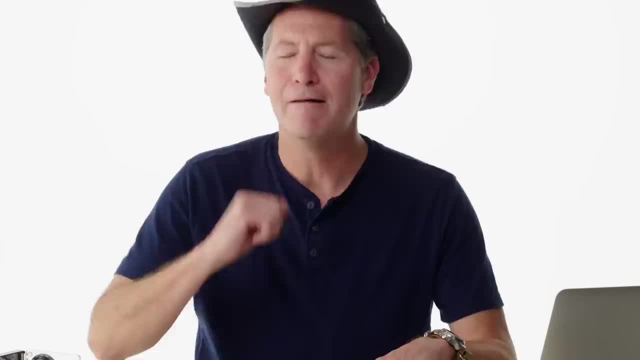 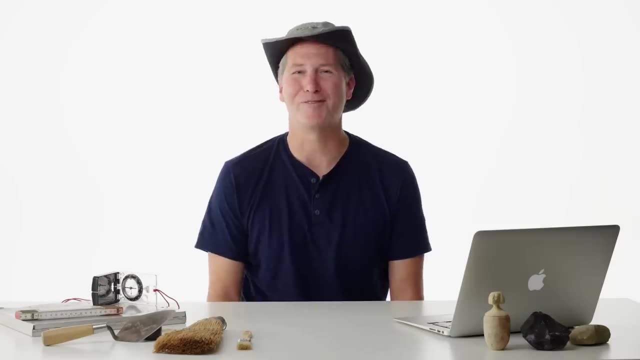 old too, 21,000 years or 40,000 years, But the evidence isn't quite good enough. A decade, maybe we know more than we do now. Those are all the questions for today. Thanks for watching. Archaeology support.